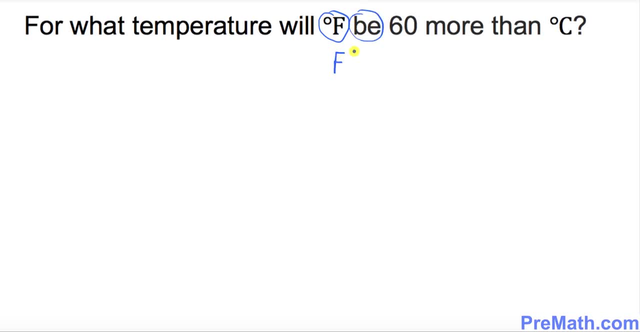 just put down F Wherever you see. B is always same as equal to 60.. Just put down 60 right up here, Wherever you see more than more than means simply plus, And then this is C. So that's all you have to put down. 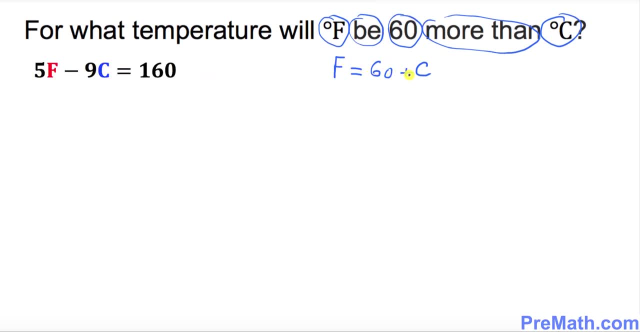 And now this is the formula that we'll be using. We got F equal to 60 plus C. Wherever you see F over here replaced by that, by substituting, So I'm going to put down 5 times: F is 60 plus C, minus 9C, equal to 160.. Let's go ahead. 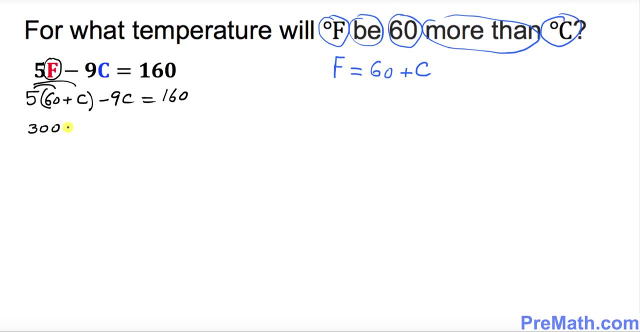 and distribute, That's going to become 300 plus 5C minus 9C, equal to 160.. So there, we got 300.. And when you simplify that become negative 4C, equal to 160.. We want to remove now this 300. So I want you to put negative 300 on both sides, So this cancels out. We got negative. 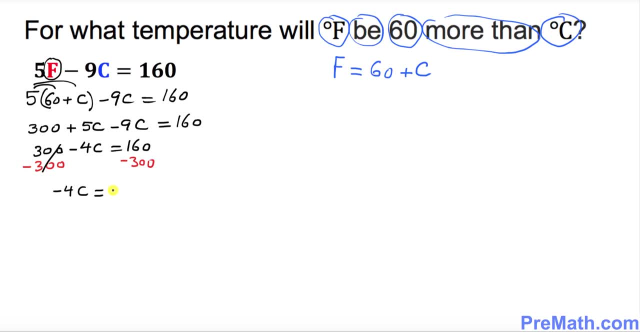 4C, equal to negative 100. And 40. I want you to divide both sides by negative 4.. So C turns out to be 35 degrees, And now we're going to find the value of F by just simply plugging in C, equal to 35. So that's going to be. 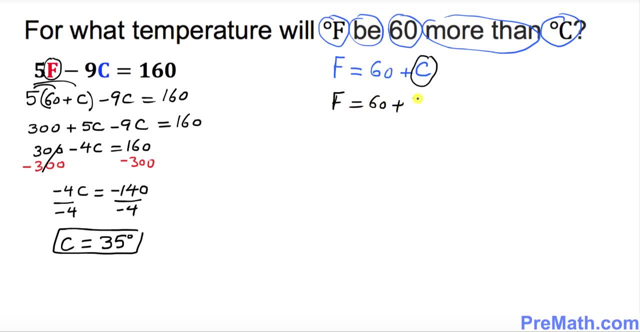 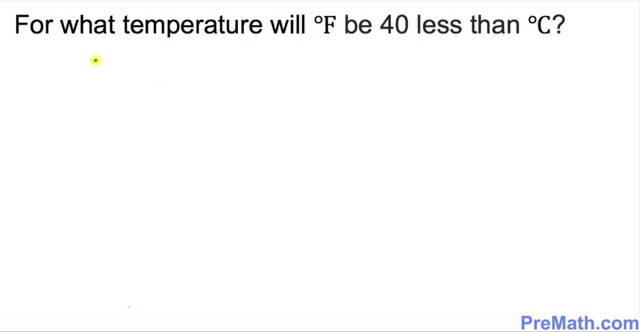 F equal to 60. Plus 35. So F turns out to be 95 degrees. So thus, at F equal to 95 degrees and C equals to 35 degrees, F is 60 more than degrees Celsius. Let's start working on the next temperature word problem right now. over here, We need to convert this one to algebraic. 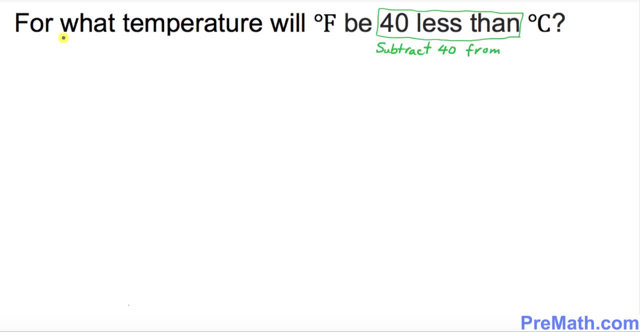 problem as well. So it says: for what temperature will degrees Fahrenheit be 40 less than degrees Celsius? Always remember in that box that I put down whenever you see less then 40. less than means subtract 40 from. So how are we going to convert into a algebraic? 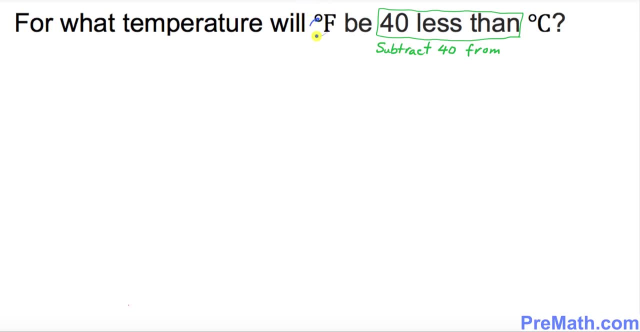 problem. Just F고. put down F as F and B is the same as tam resist, as 곧 menos 40 Academy – Summa Cumlude, When you see, less then mean subtract 40 from to 40. less than means subtract 40 from, so it's going to be a C minus 40 always. 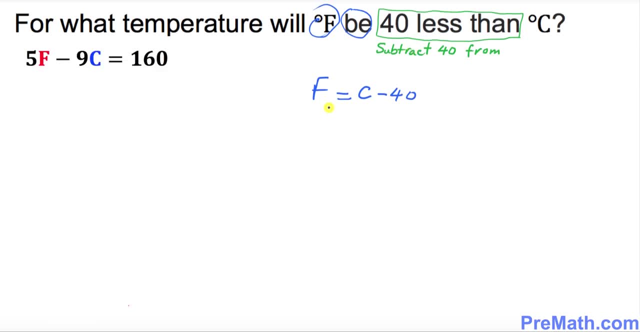 remember C minus 40. so now this is the formula that we will be using and F equal to C minus 40. so I'm gonna replace F by C minus 40. so I'm going to put down five times C minus 40 minus 9 C equal to 160. let's distribute that one, so 5 C. 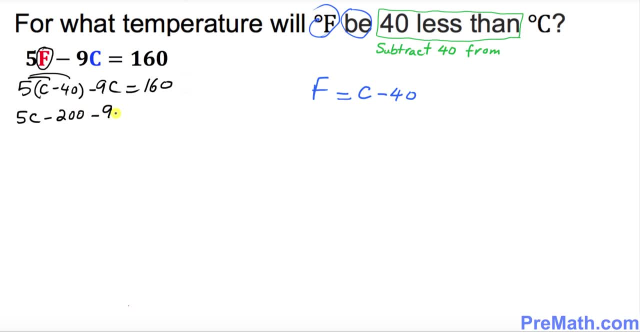 minus 200 minus 9 C, equal to 160. so 5 C minus 4 C is 9 C is negative. 4 C minus 200, equal to 160. now i want you to remove this 200 to other side, so i'm gonna add 200 on both sides. 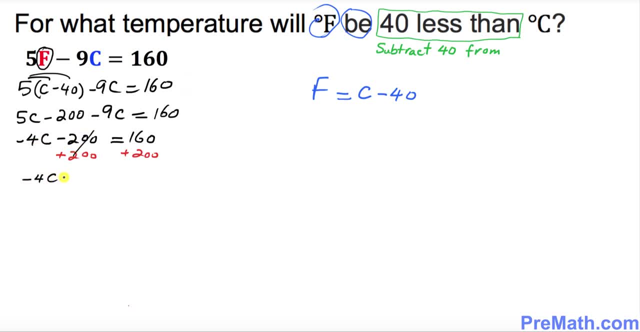 this cancels out. so we got negative 4. c turns out to be equal to 360. i want you to divide both side by negative 4, so c turns out to be negative 90 degrees. now we're going to plug it back over there wherever we got c equal to negative 90 degrees right up here. so f equal to negative 90. 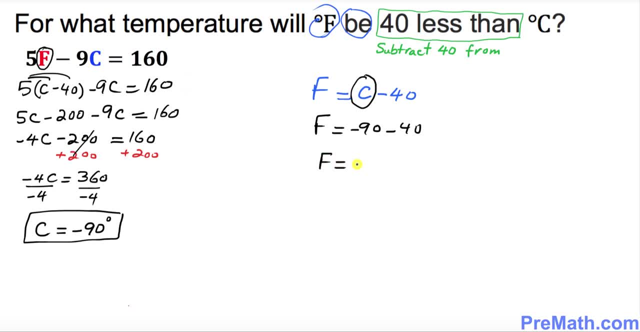 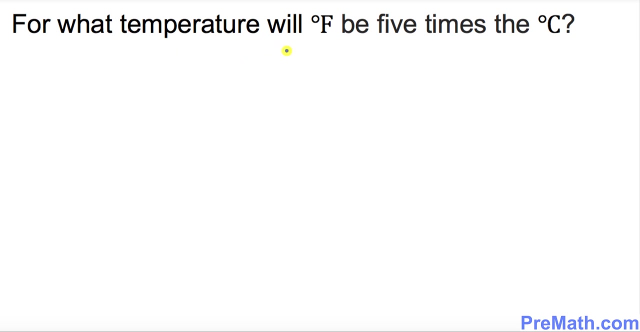 minus 40, so f turns out to be a negative 130 degrees. so thus f equal to negative 130 degrees and c equal to negative 90 degrees. f is 40 less than degrees celsius and finally, we'll be working on this word problem- this is for what temperature will.